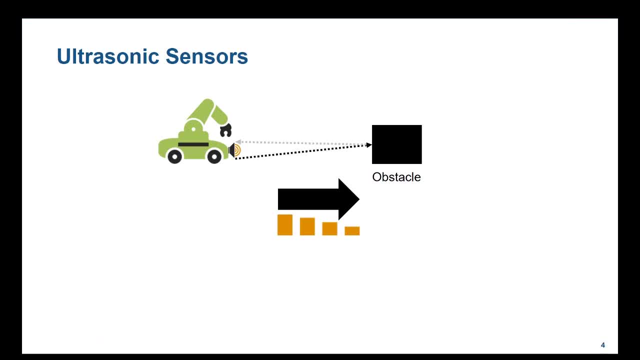 Ultrasonic sensors usually have three important values that characterize them. The first one is called the maximum range. This tells what is the farthest distance that the sensor can measure. The second value is called the minimum range, And this tells what is the minimum distance that the sensor can measure. 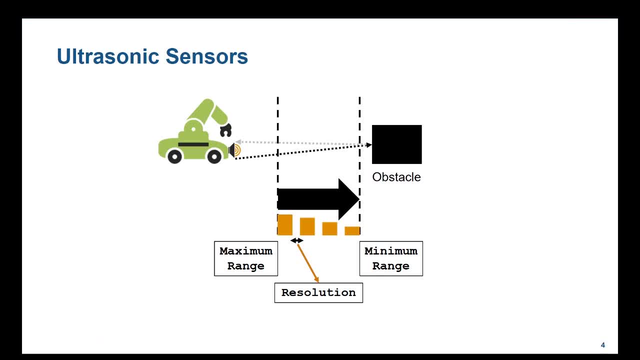 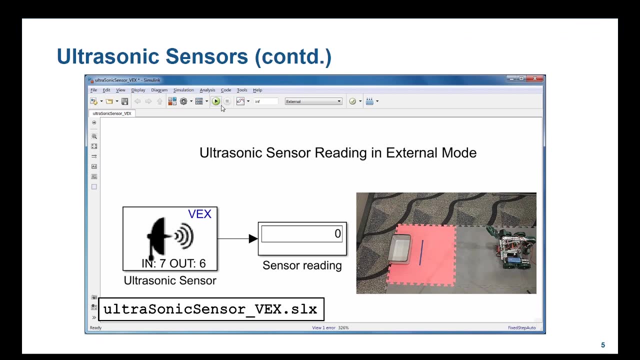 The last value is called the resolution, And this tells us what is the smallest change that the actual ultrasonic sensor can detect. We can note down all these values from data sheets or by using experiments. Let's take a look at a video of an actual robot to understand these sensors. 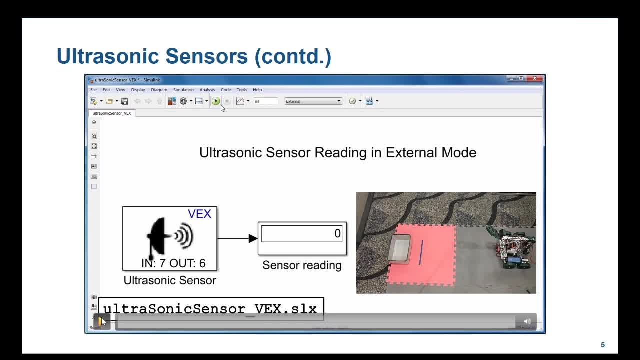 Here is a sensor in front of the robot. We are looking at the robot in front of us. We can see the value returned by the sensor. This is the closest obstacle that it can see, In this case the basket. The sensor value starts around 0.8 meters and, as the robot is manually moved slowly, 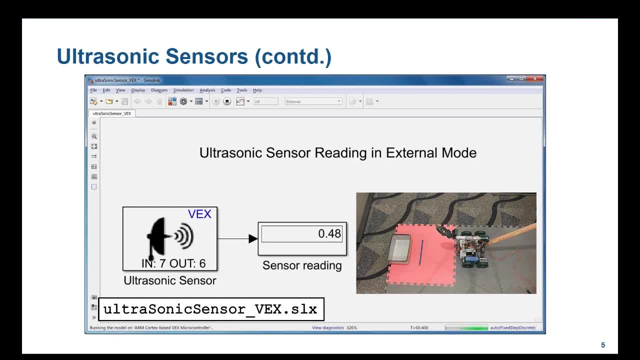 the value keeps decreasing, This is because the robot is approaching the obstacle. We can also see some zero values intermittently. Sometimes sensors could drop values and this scenario needs to be considered when building the algorithm Towards the end. the sensor shows 0.02, even when the sensor is literally touching the obstacle. 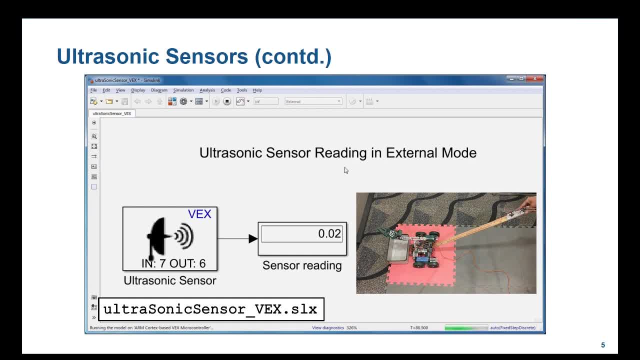 This is the characteristic of the sensor, since it can only measure 0.02 meters as the minimum distance, This is also called the minimum range of the sensor. Let's note these values from the data sheet here. So the maximum range is 2 meters. 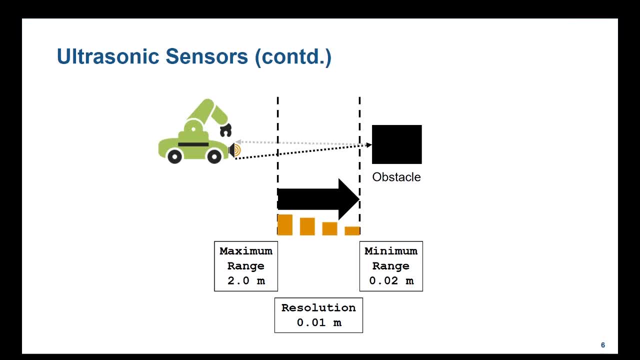 The minimum range is 0.02 meters And the resolution is 0.01 meters. These values were noted from the data sheet for the VEX platform. These values were noted from the data sheet for the VEX platform. Now that we have understood the characteristics of the real sensor, 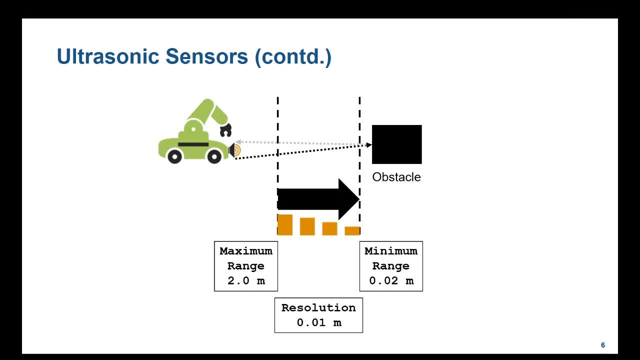 Now that we have understood the characteristics of the real sensor, let's see how to bring this information into our simulation. let's see how to bring this information into our simulation. In the real world, the robot travels over the map and the ultrasonic sensor provides us with a value corresponding to objects in front of it. 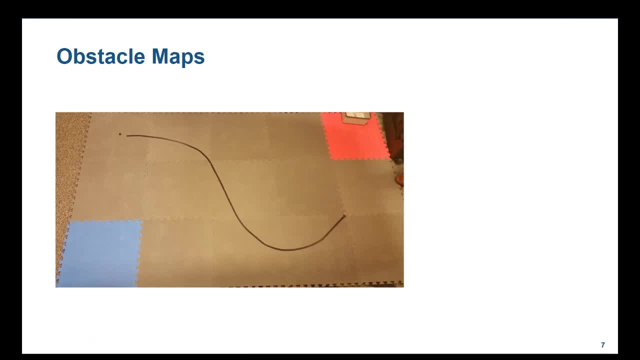 In the real world, the robot travels over the map and the ultrasonic sensor provides us with a value corresponding to objects in front of it. In the real world, the robot travels over the map and the ultrasonic sensor provides us with a value corresponding to objects in front of it. 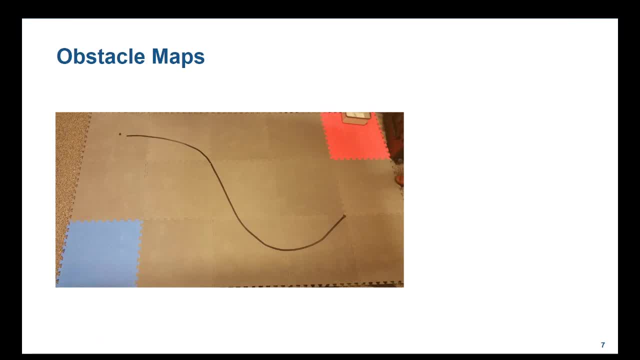 In the real world, the robot travels over the map and the ultrasonic sensor provides us with a value corresponding to objects in front of it. In the real world, the robot travels over the map and the ultrasonic sensor provides us with a value corresponding to objects in front of it. 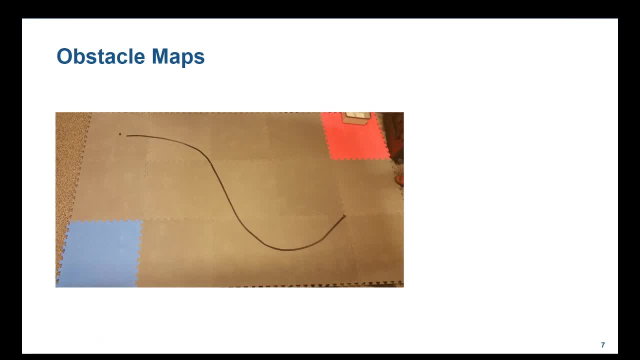 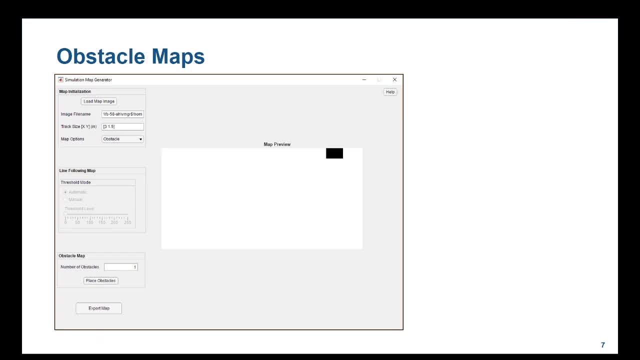 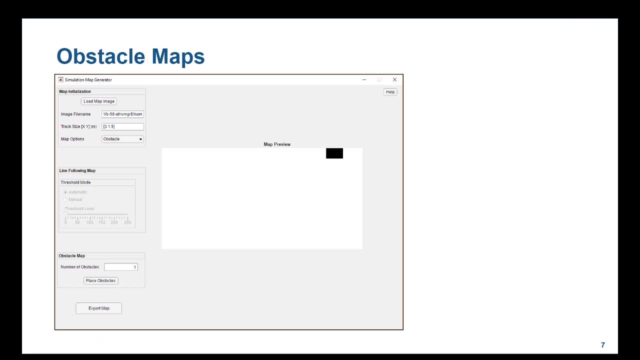 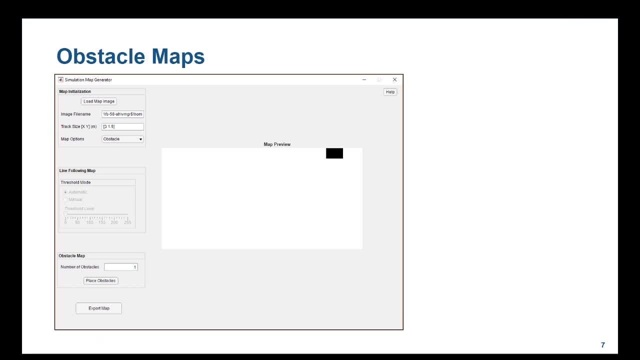 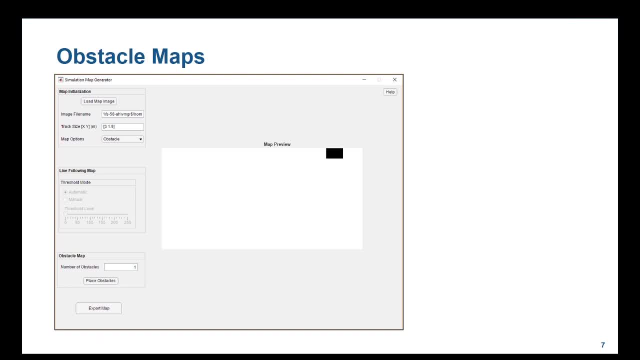 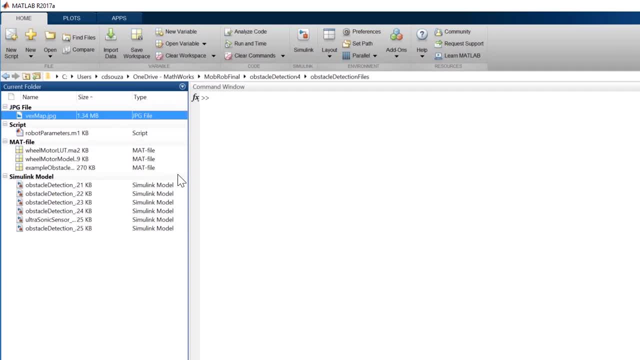 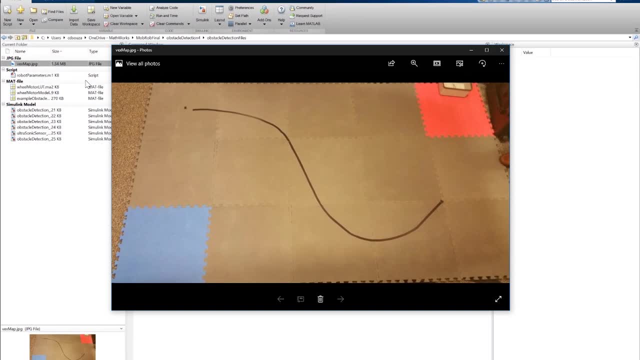 Let's switch to MATLAB to see how to do this. On the left side of the map you can see a picture called WexMapjpg. Let's open this outside MATLAB to see that it is the path we are trying to navigate. Our objective will be to place obstacles in the region of interest. 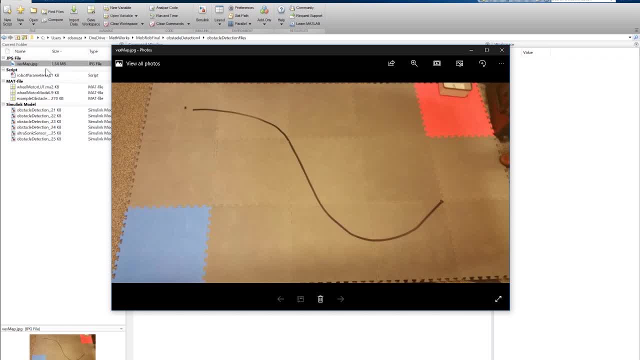 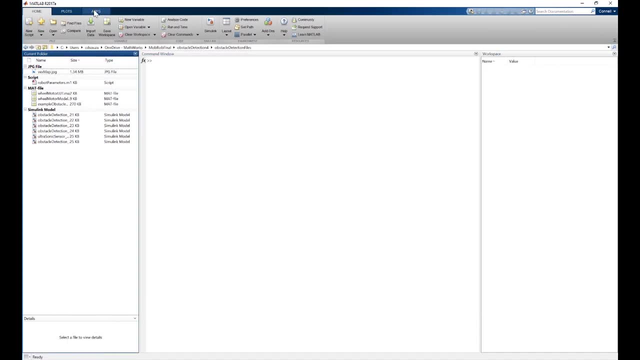 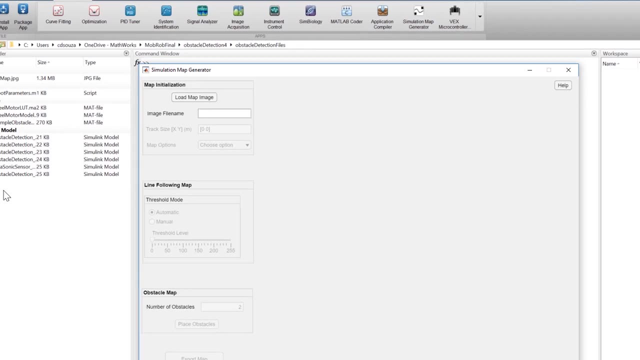 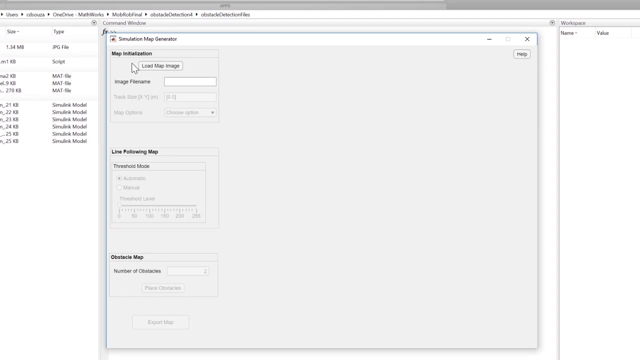 In our case, we have only one obstacle, So let's use a simulation map generator. Let's go back into MATLAB tab. let's choose the simulation map generator. The first step is to load the picture which can be used as a reference to place the obstacles. So let's click on. 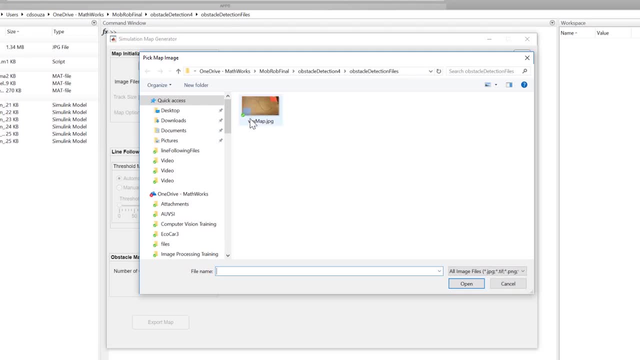 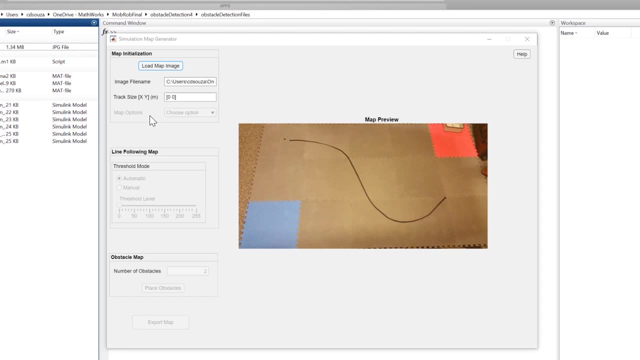 the load map image button and let's select the VEXMAPJPG image. This pulls up a preview of the image on the right-hand side of the interface. Next we need to specify the size of the map, in meters where X is along the horizontal. 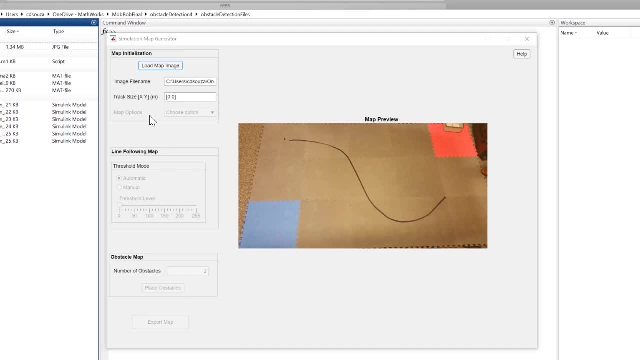 axis and Y is along the vertical axis. Using a tape measure, we determine this for our map to be 3 and 1.5 meters, So let's insert it right here. Hitting enter enables the next option. Now we need to specify what type of map we're trying to. 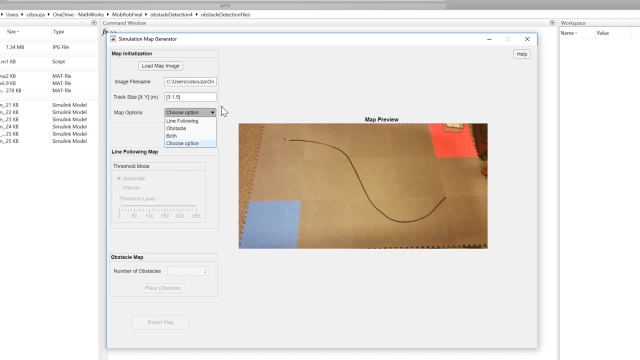 generate. Since we are only concerned with obstacle detection in this video, let's choose the obstacle option. We talked about line following maps in the previous video. If the robot is trying to perform both line following and obstacle detection, then the both option might be. 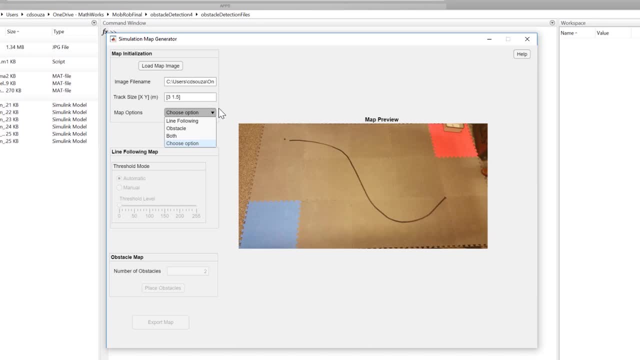 useful. We will see how to do this in the next video, So let's choose the obstacle option for now. As soon as you select the obstacle option, the preview changes to a blank white image. This means that currently there are no obstacles on the. 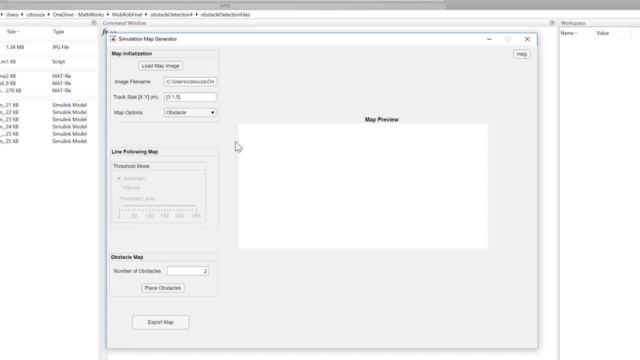 map. The idea is to place obstacles on this map so that obstacles look blank and everything else looks white. So first we need to specify how many obstacles we would like to place on the map. The default option is 2.. We can change this to 1, since we only have one obstacle in our map, just like I'm. 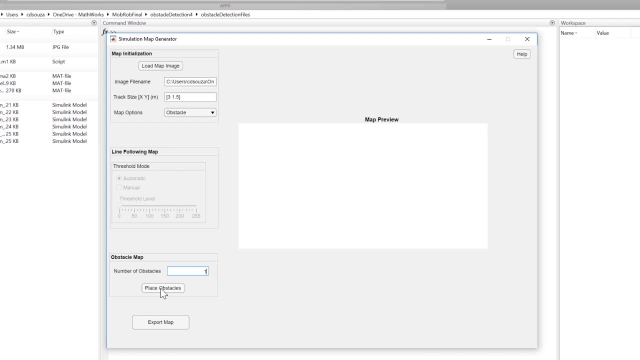 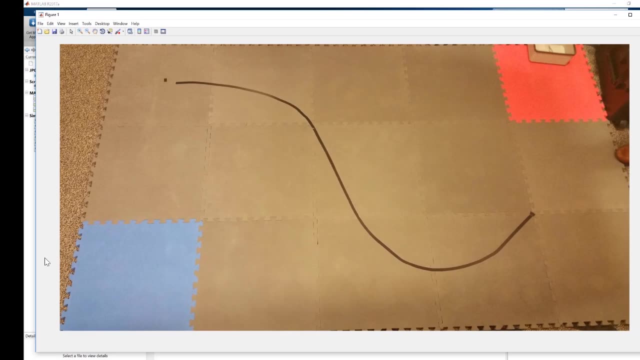 doing over here. After setting this value, hit the Place Obstacles button. This opens a new window with the original map picture. To place the obstacles, click and draw a rectangle in the image over the region of interest, just like I'm doing right here Once the region of interest. 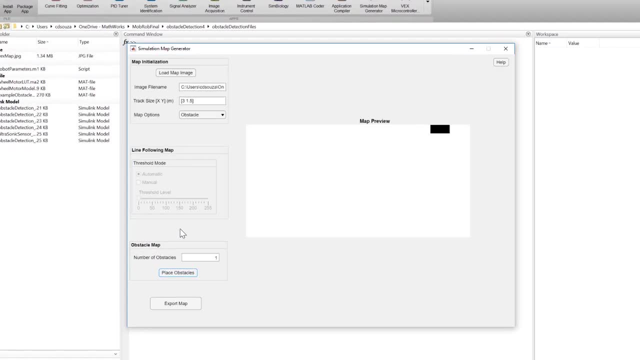 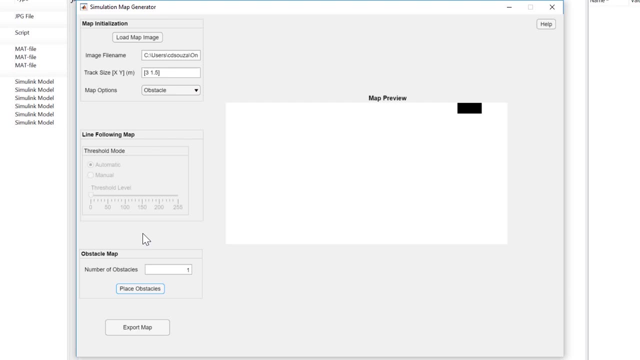 has been selected, double click inside the region and now we can see that the obstacle has been placed in the map preview. We will use this map for our obstacle detection simulation. If we have more than one obstacle, we can simply change the number of obstacles appropriately and repeat the obstacle. 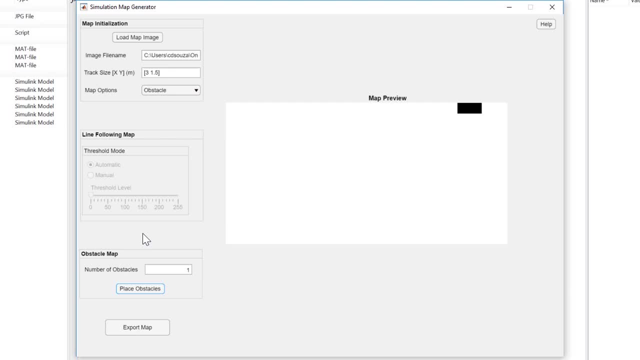 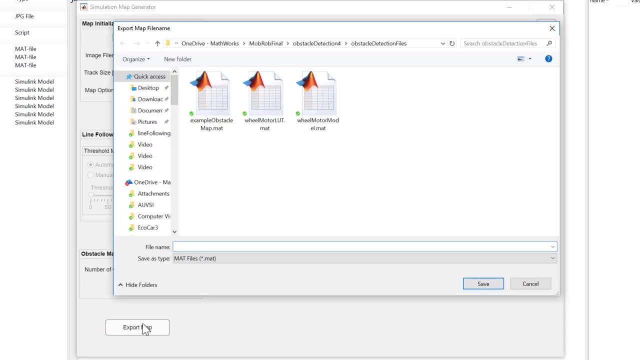 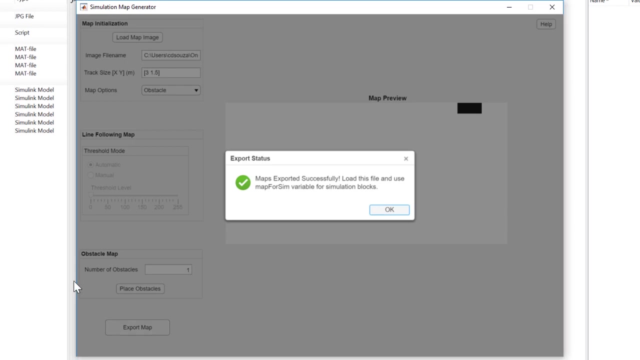 placement process for each of the obstacles. Once the preview looks acceptable, let's hit the export map button and let's give it a valid name. So let's call it obstacle map and let's hit save. Once the file is saved, we see a success message. We can now load the file that we've just exported and use it for. 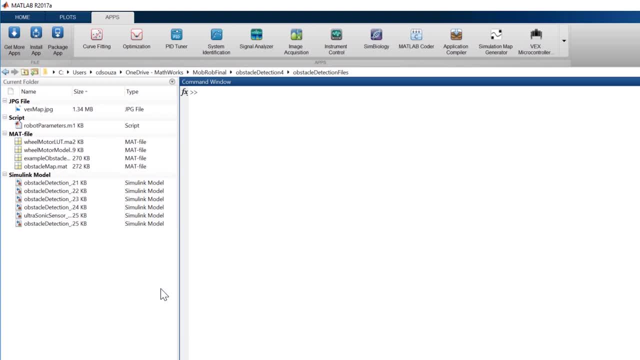 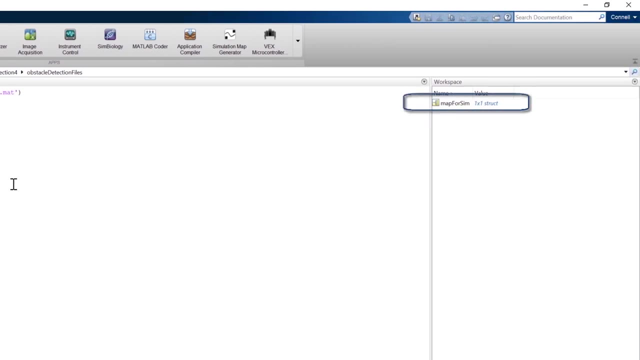 simulation. To do this, let's go back to MATLAB and double click on the obstacle map dot mat file that has been created in the current folder, So let's double click on it. This and this creates a variable called map for sim in the MATLAB workspace. We 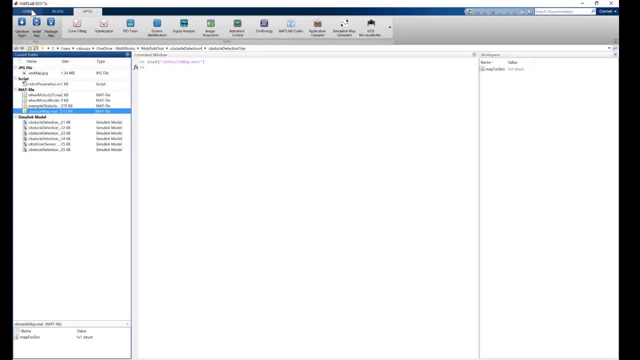 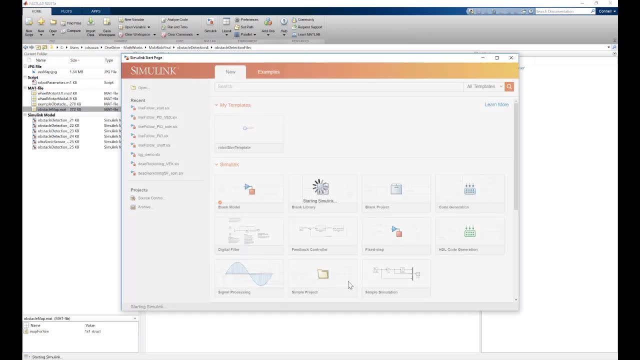 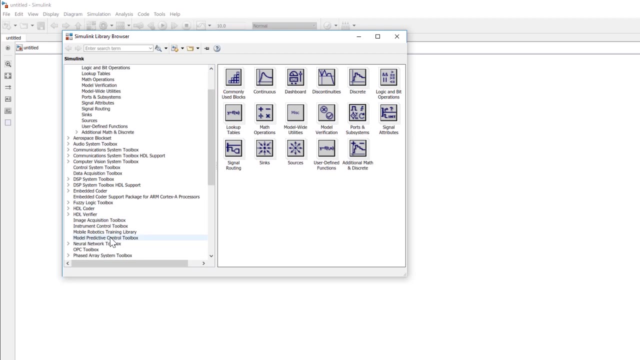 can use this variable for our simulations. To set up our obstacle detection simulation, let's open a new Simulink model, Let's go into the Simulink library browser and from the mobile robotics training library, let's add the ultrasonic sensor to the model. 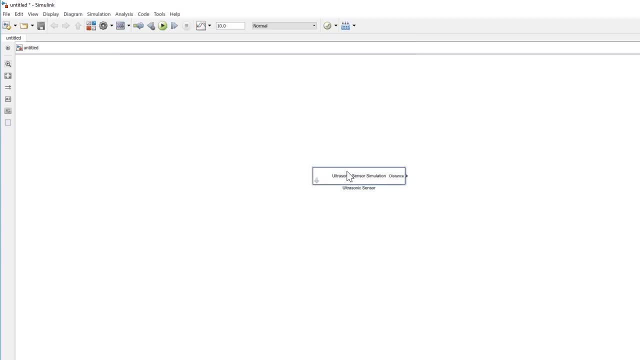 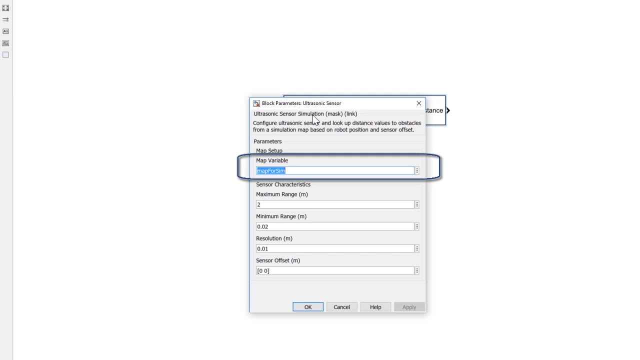 This block will represent our real ultrasonic sensor. Let's double click on the block to set up its parameters. We see that the map variable has already been set as map for sim. This is the variable we just loaded in MATLAB. Apart from this, we can also specify sensor characteristics. For example, we 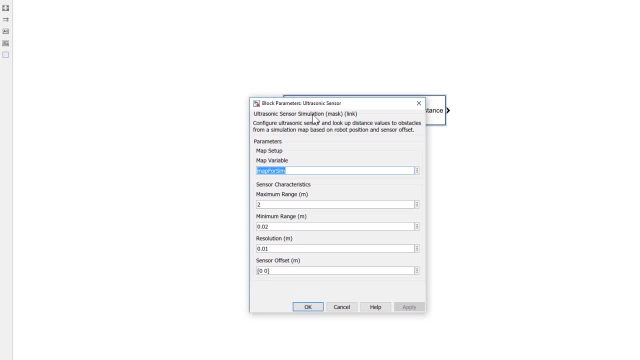 use data sheets to find values for the range and resolution of our sensor. We can specify these values here to make the block output values like the actual sensor we are trying to model. We can also specify a sensor offset here that specifies where the sensor is positioned with respect to the center of 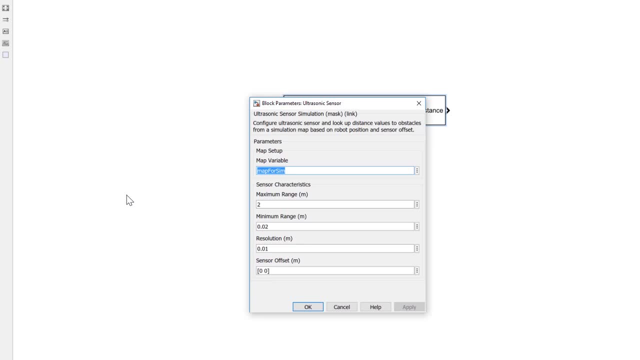 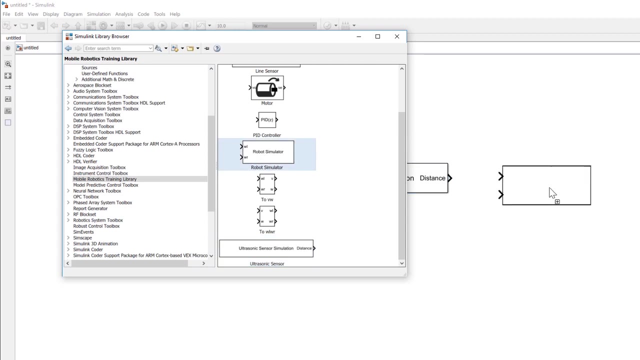 the robot. Let's leave it as 0,0 for now. Let's hit OK. Now, going back to the mobile robotics training library, let's add the robot simulator block into the model and let's double click on it to set up its parameters For the 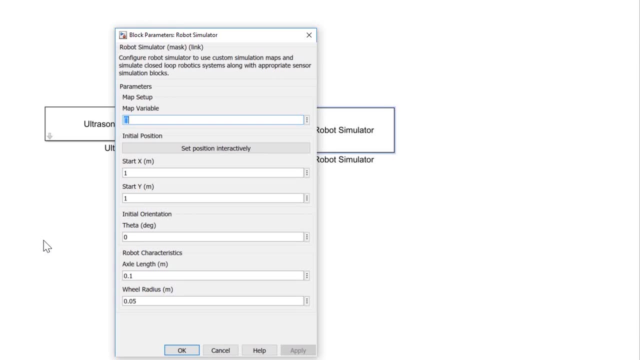 obstacle detection simulation. like in the line following simulation earlier, we need to set the map variable to map4sim. So let's go ahead and do that And recall that map4sim is a variable that we just created in the MATLAB workspace. Once we specify the variable, let's hit apply. This brings up another. 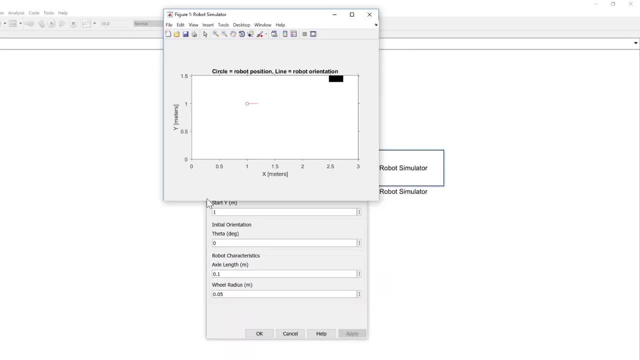 window with the updated map. Note that the robot starting position is 1,1 here. If you wanted to specify it to be anywhere else interactively, let's go back to the parameter dialog and choose the set position- interactivity. This brings up another window of the map. You can double click on the. 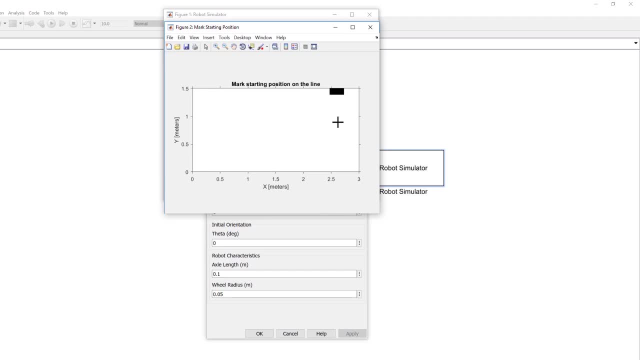 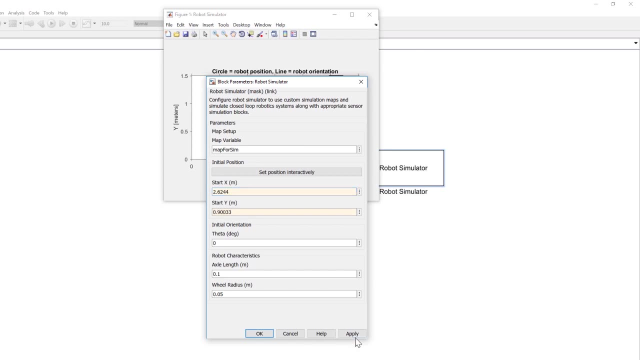 point that we want to set the position to. So let's double click here, and now we see that the position has been updated in the parameter dialog. Now let's hit the apply button again, and now we can see that the robot has been put at the. 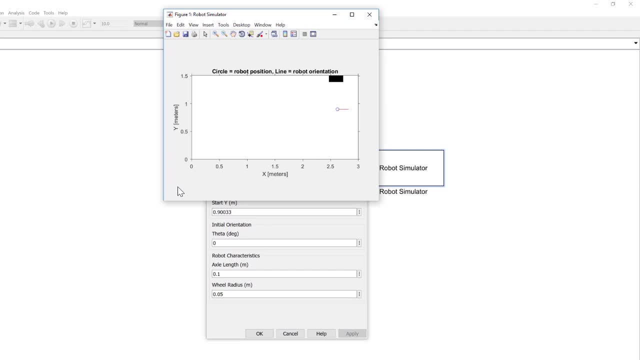 starting position that we just selected. However, the robot is facing towards the right. We need to position it such that it is pointing in the upwards direction. So let's set the initial theta value to 90 in the parameter dialog and now let's hit apply again. Now our robot is. 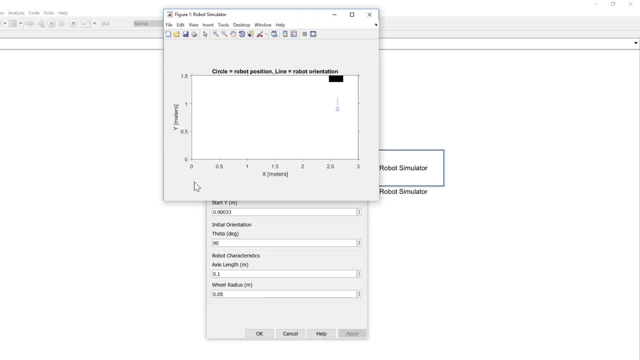 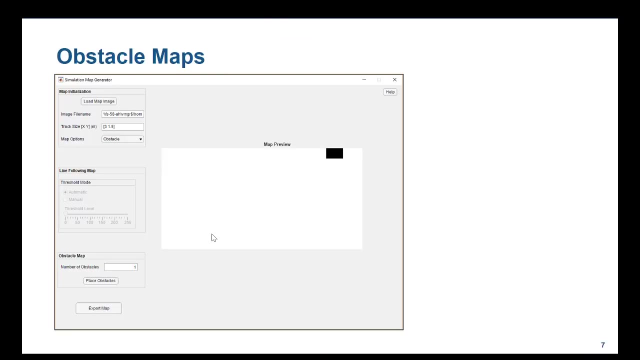 facing the obstacle and we can implement our obstacle detection algorithm to see if we can find the obstacle at an appropriate distance. Let's go back to the presentation and do a short recap. To set up an obstacle detection simulation, we began with the simulation map generator. We loaded an image of the map. 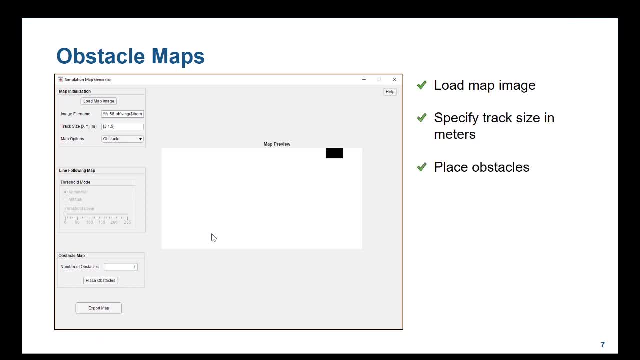 and then specified the track size for the obstacle detection map. We then talked about placing obstacles interactively, so that the obstacles look like black rectangles on the map and everything else is white. finally, we exported the map to a mat file. we then loaded the mat file. 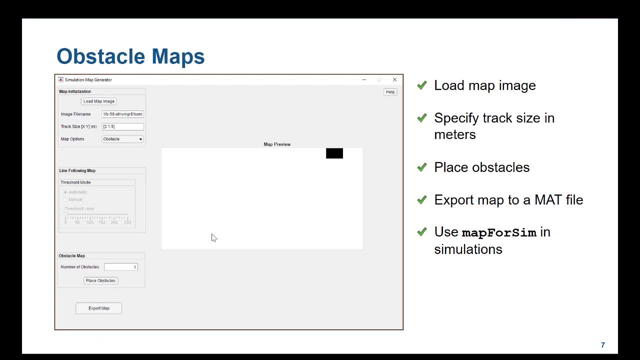 and saw the map for sim variable to be used for simulation. we have specified this variable in the ultrasonic and the robot simulator blocks. here are some of the best practices to use the simulation map generator for obstacle detection simulation. make sure the track size measurement is accurate enough. this directly affects how the distance measurements are made in the map. 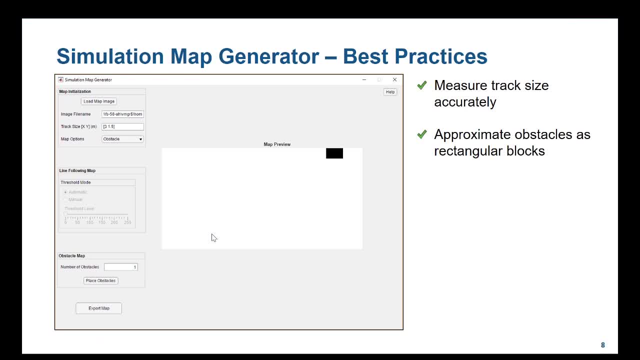 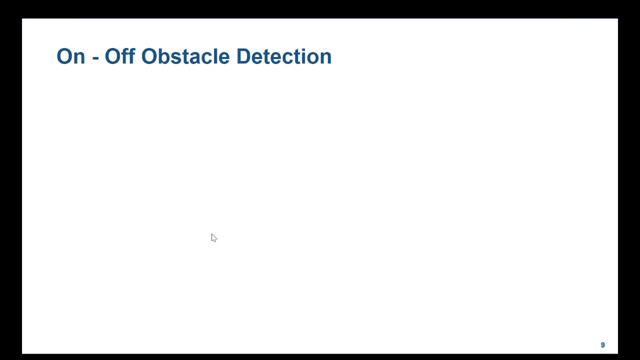 also approximate obstacles as rectangular blobs. now that we have set up the simulation, let's implement an obstacle detection algorithm and see it in action. one of the more popular obstacle detection algorithms is called the on off algorithm. the basic logic for this is as follows: we first check the value returned by the ultrasonic sensor. 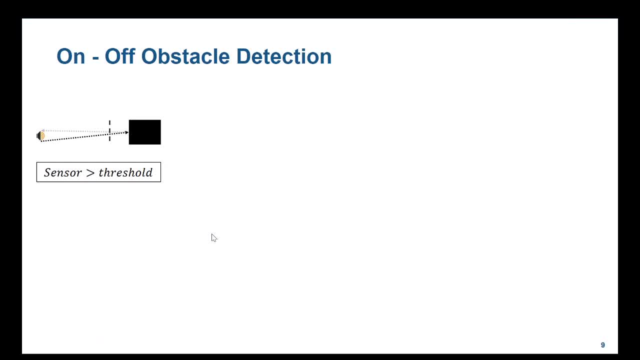 if it is greater than a threshold, then the robot is still a distance away from the obstacle. we must keep going forward towards the obstacle. if the sensor value is less than the threshold, that is, the robot is within the threshold distance from the obstacle- we must stop. let's put this logic in a flow chart format to better understand the algorithm. 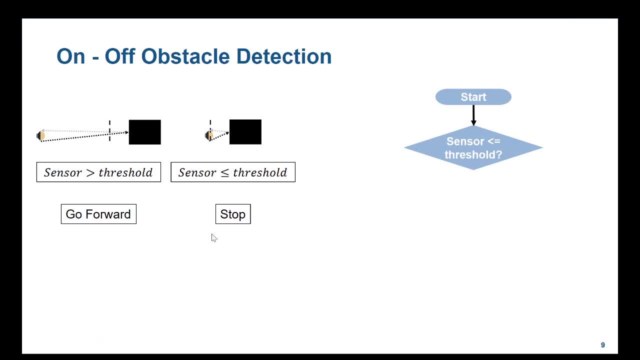 we first check if the sensor value is within the threshold value. if not, we keep moving forward, else we stop. since the algorithm has only two states that it can move between, it is called an on-off algorithm. let's switch to matlab to see how we can do this. let's open the startup model: object detection- underscore- start. 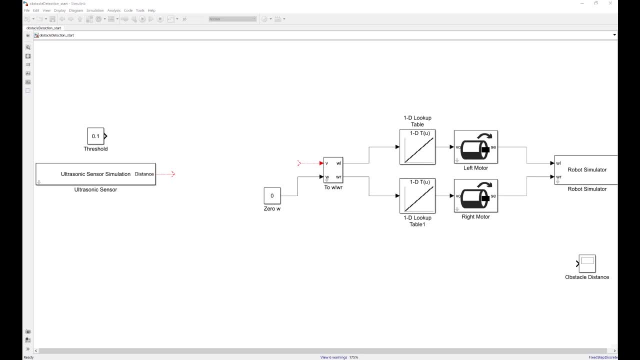 the model already has several blocks. to start with, notice the ultrasonic sensor and the simulation simulator block that we set up earlier in the video. it also has blocks that we have already talked about in previous videos, namely the motor, the and the lookup table blocks. our goal is to now. 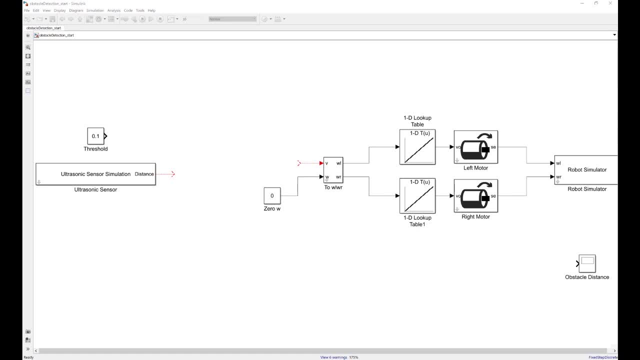 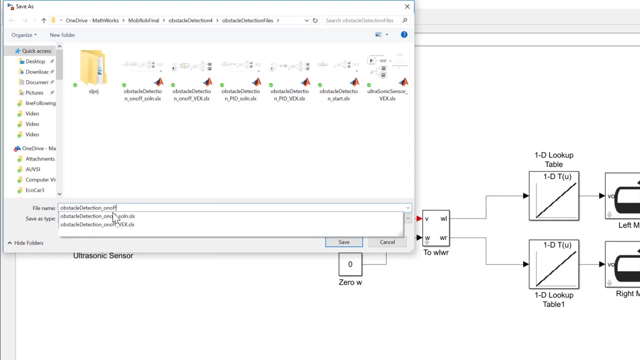 use the ultrasonic sensor information to generate the linear velocity v value to help the robot stop 0.1 meters away from the obstacle. so let's use state flow for this. let's start off by saving the model as obstacle detection underscore on off and let's hit save from the simulink library browser. let's add a state flow chart to the model. 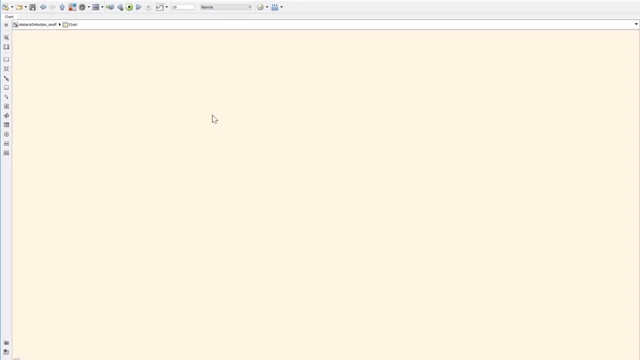 and now let's double click on the state flow chart to define the logic. just as we discussed in our flow chart before, there are two states in an on-off algorithm. so to add a state, click the state option on the toolbar on the left and drag it into the model. 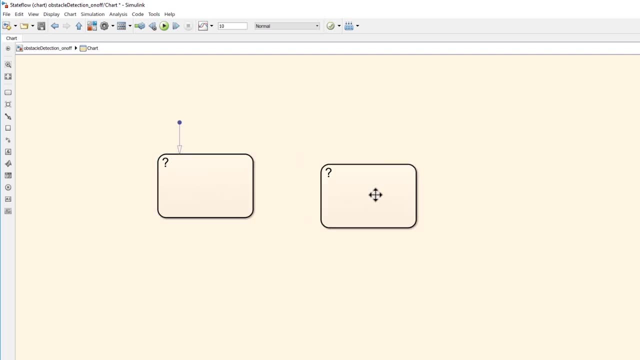 you can copy a state in the same way that you copy simulink blocks, by right clicking and dragging. so now we have two states. let's call the first state the go forward state and the second state the stop state. our robot will go forward by specifying a constant velocity value, for example v. 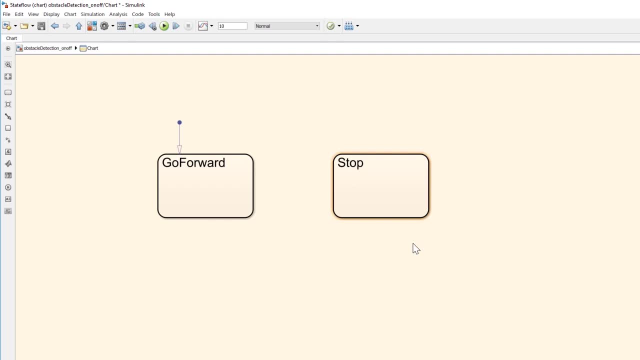 equals 0.2, and for the stop state we will set up a level without propellants, with the same state value, the same V value to zero. So let's define the logic: In the go forward state we set V equals 0.2 and in the stop state we set V equals zero, Since our algorithm can shuttle between these. 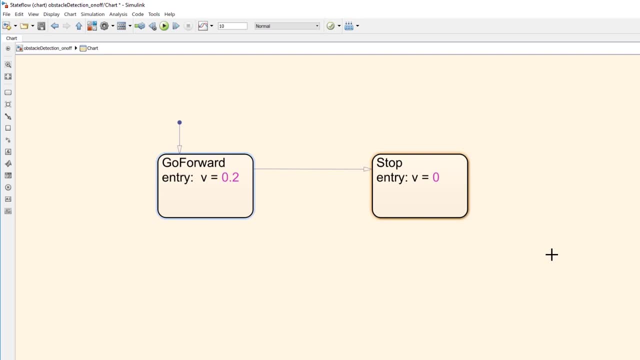 two states. let's connect them with the back and forth connection, just like we did in the previous videos. Next, we need to define the condition that will decide moving between these two states. So we know that when the ultrasonic value is less than or equal to the threshold. 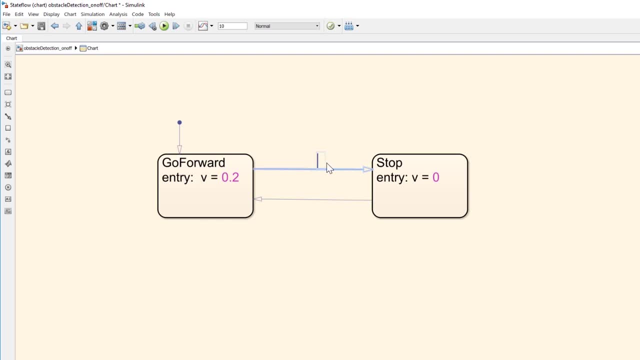 it will move from the go forward to the stop state, So let's define that. And when the ultrasonic value is greater than the threshold, it will move from the stop state to the go state, So let's define that as well. So let's resolve the symbols in this chart. Recall that to resolve the. 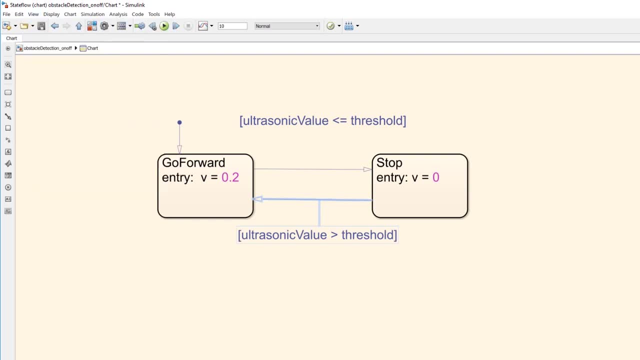 symbols in this chart. we need to define the condition that will decide moving between the symbols. you go to the view tab and choose the symbols option, which pulls up the pane on the right hand side of the screen. You can resolve the symbols by clicking on this exclamation mark up. 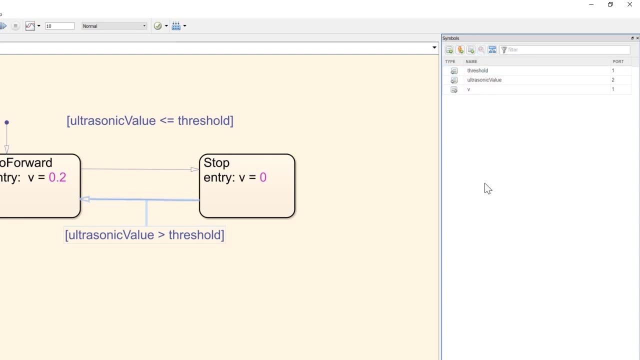 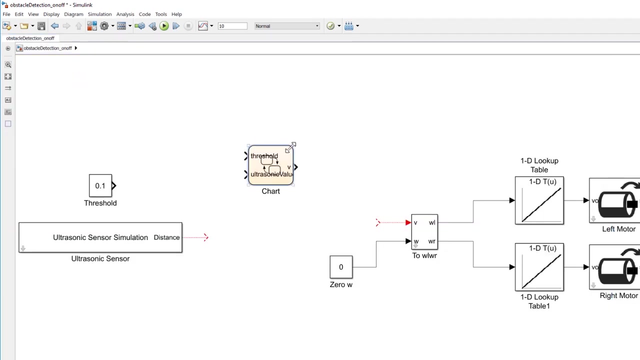 here, And now we can see that threshold and ultrasonic values have been set as inputs and V has been set as an output. The next thing to do would be to go up one level in the model and connect the ultrasonic block to the input of the chart. So, as you can see, 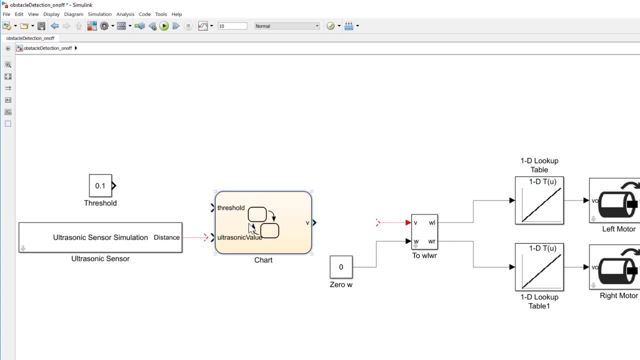 we've got two inputs and one output to the chart, And the ultrasonic sensor will connect to the ultrasonic value input And the V value will connect to the utility block. Now the threshold is the reference distance from the obstacle, So let's connect the threshold. 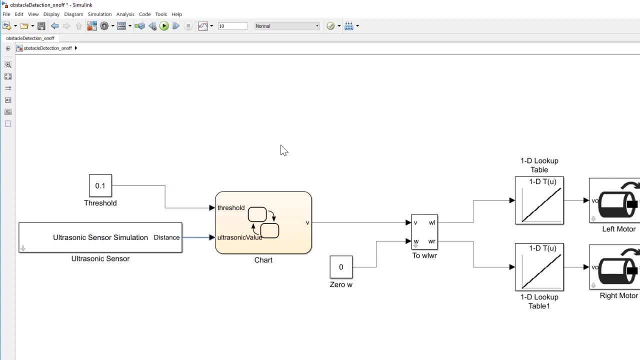 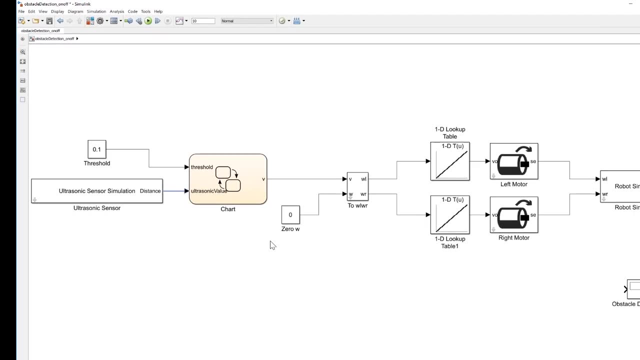 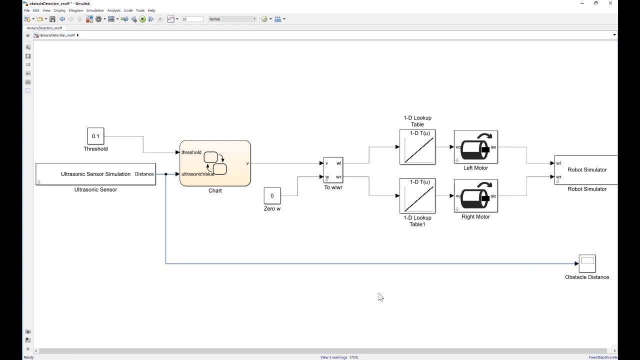 constant block to the input of the chart And notice that, since we are only moving in a straight line, the omega value has been set to zero using the zero omega constant block. Let's also connect the output of the ultrasonic sensor block to the obstacle distance scope over here. 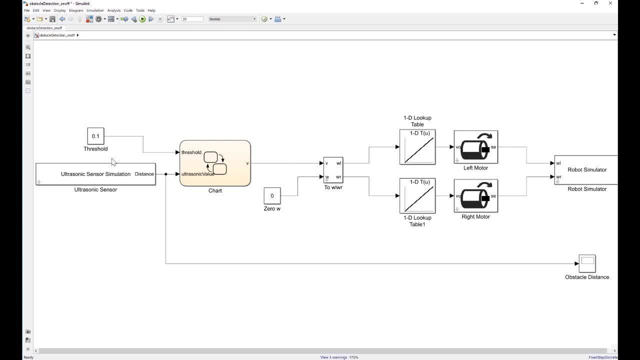 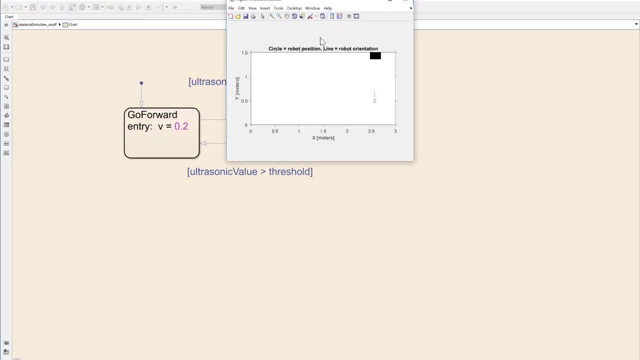 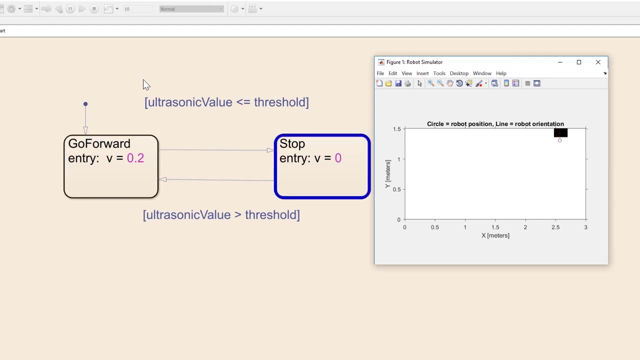 This will help us visualize the ultrasonic sensor data. Let's go back into the state flow chart and let's run our model. We see that the robot moves in a straight line and stops just before the obstacle. In the chart we can also see that the state's shuttling from the go forward to the stop state. Let's go back. 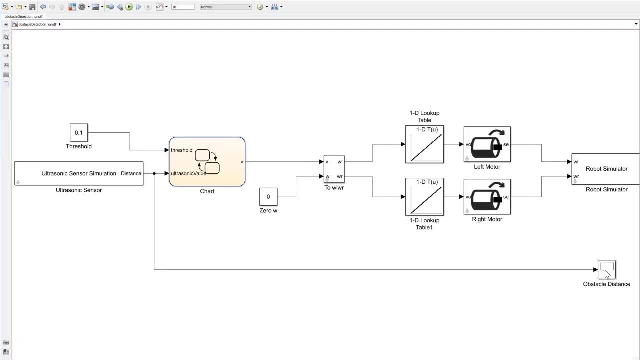 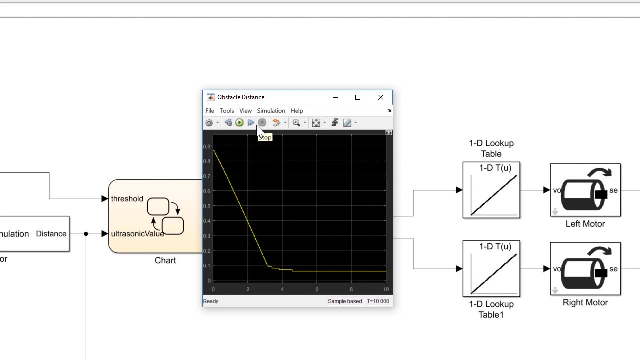 up to the top level of the model and view the obstacle distance scope, We can see that the robot moves towards the obstacle and stops when the obstacle is a little less than 0.1 meters away. Note that the distance value goes below 0.1.. 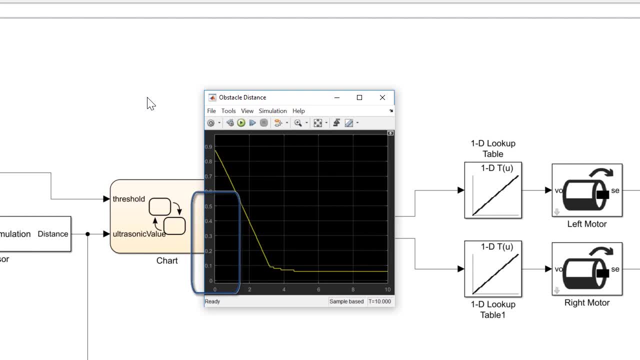 This is because we are asking the robot to stop immediately from a velocity of 0.2 to zero, which is not physically possible. This results in the robot going below the the threshold value and we can see a staircase like response. This is because of the way in. 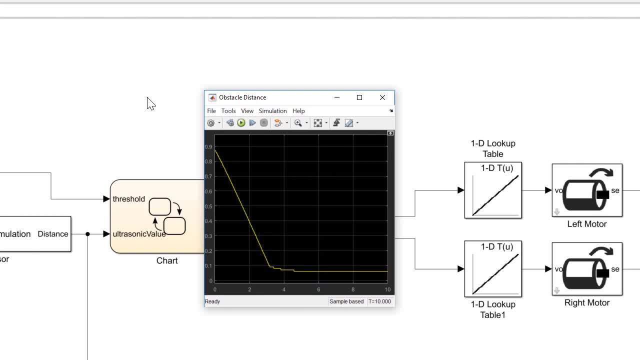 which we model the sensor using a resolution parameter, which is the minimum distance that it can see. Now we use this simulation to test the obstacle detection algorithm. Let's look at how the actual robot performs with this algorithm. Let's go back to the presentation. 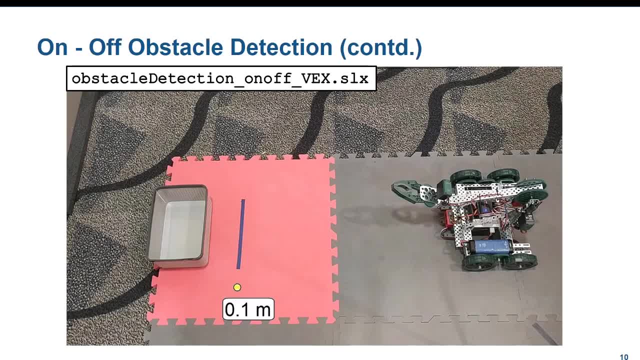 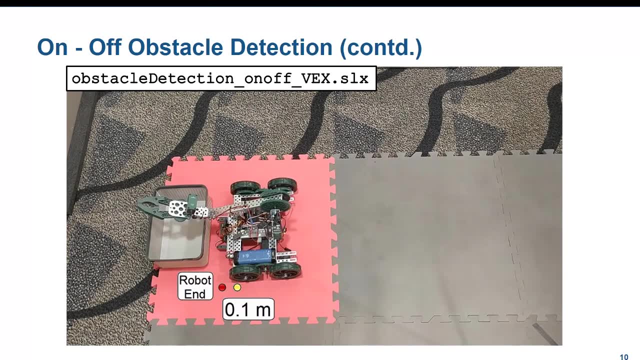 We just saw how to implement the on-off obstacle detection algorithm. We see that the robot went beyond the line that signifies the 0.1 meter distance to the obstacle. Our simulation showed a similar result. The advantage of this algorithm is that it is simple to implement The result. 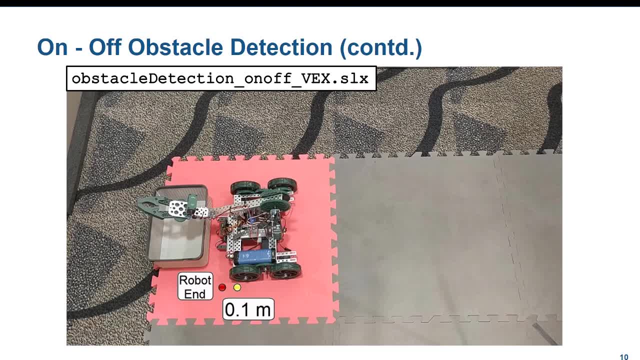 could be inaccurate, based on how fast the robot is traveling. We can achieve smoother and a more accurate stop for obstacle detection using the on-off obstacle detection algorithm, PID control. Let's see how to do this. next, Here we have our robot that is actuated by the motors. 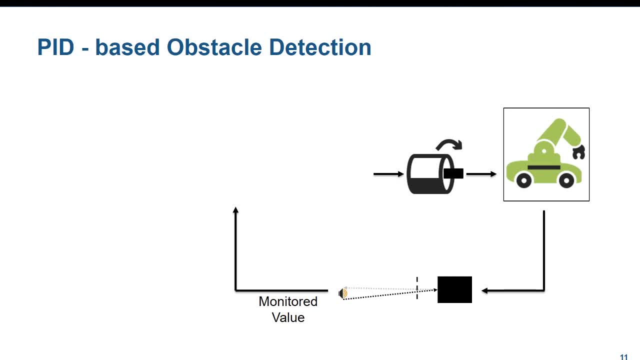 Using an ultrasonic sensor, we can monitor the current distance to the obstacle. We can then compare this with a desired reference value. This is the threshold value that we talked about during the on-off discussion. Using these two values, we can calculate an error. This error can be fed into the 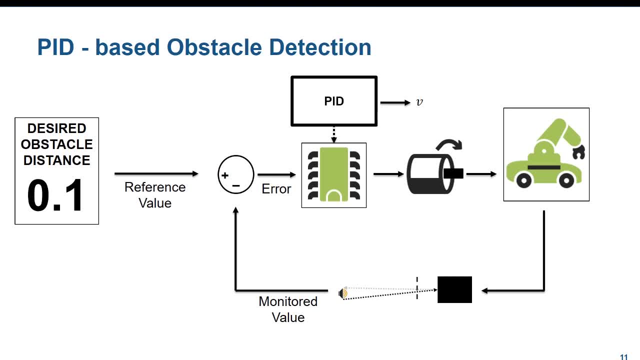 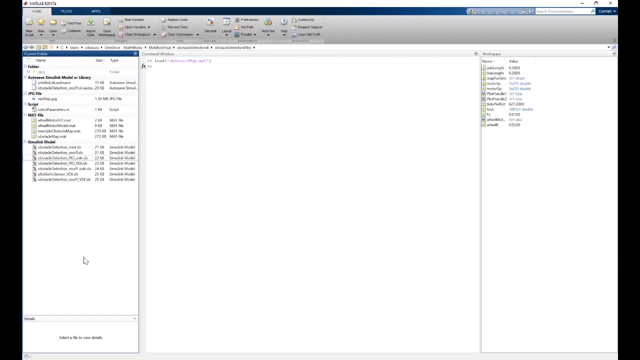 robot's speed to the PID controller. Note that the PID controller outputs a velocity v value based on the input error. The omega value is still 0. since the robot is moving forward in a straight line, Let's switch to MATLAB to see how to implement this. 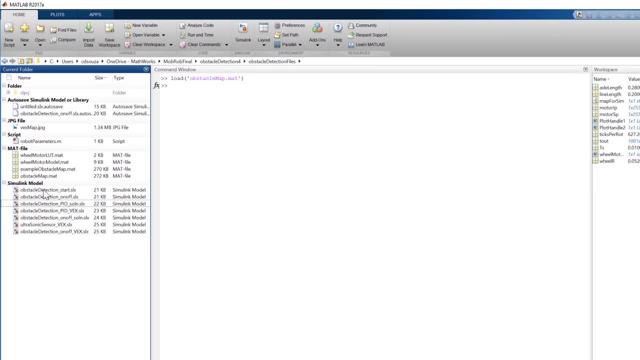 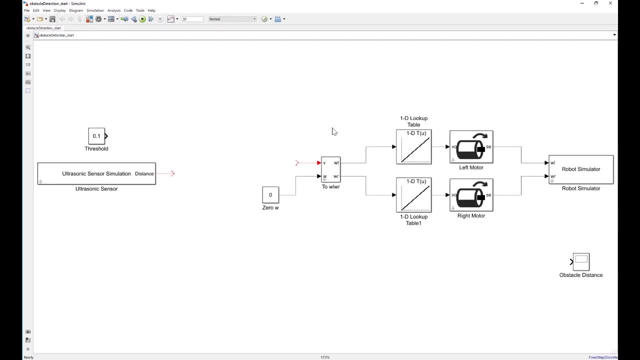 Let's open the starter model obstacle detection underscore. start just like we did earlier. Our goal is to use the ultrasonic sensor information to generate the v value to help the robot start Now. the robot is moving forward with the speed of the robot. Let's add the PID controller. 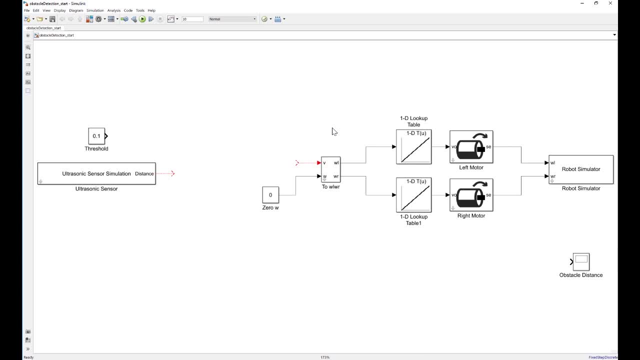 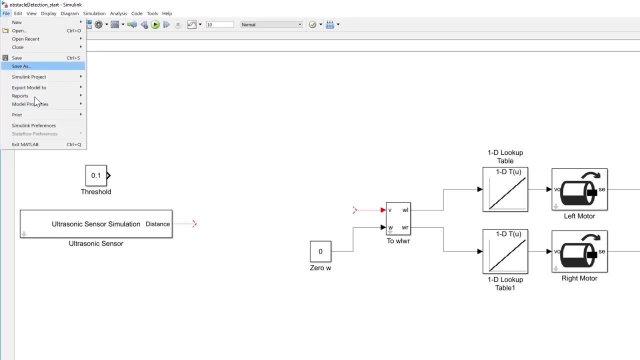 The robot is moving now. It will be solved soon. We will see the robot when it is ready. stop 0.1 meters away from the obstacle. We will use a PID for this. Let's save this model as obstacle detection underscore PID. 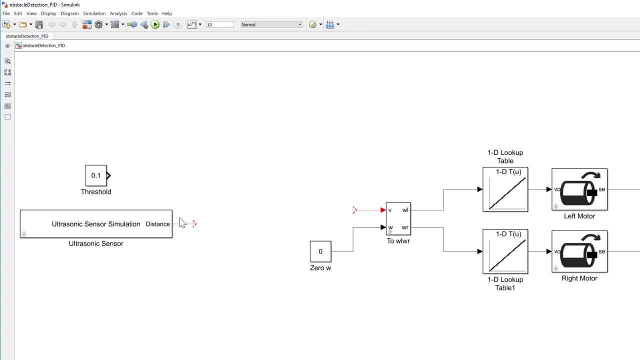 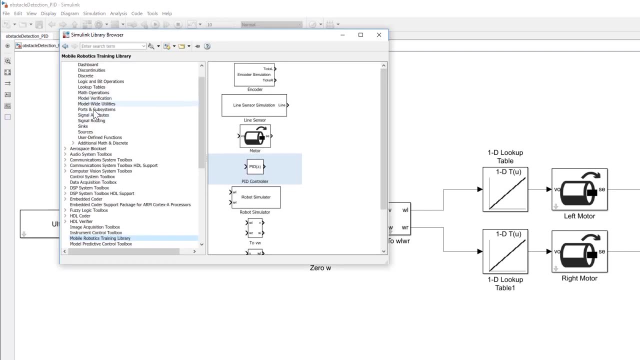 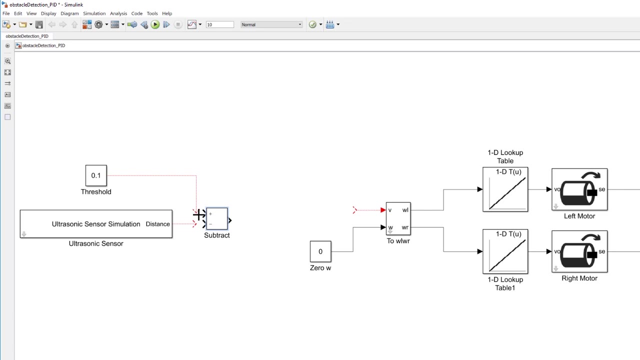 Now. first we need to compute the error between a desired value and the actual value. So let's add a subtract block to our model from the math operations library in the Simulink library browser. Now our desired value is the threshold, so let's connect that to the positive. 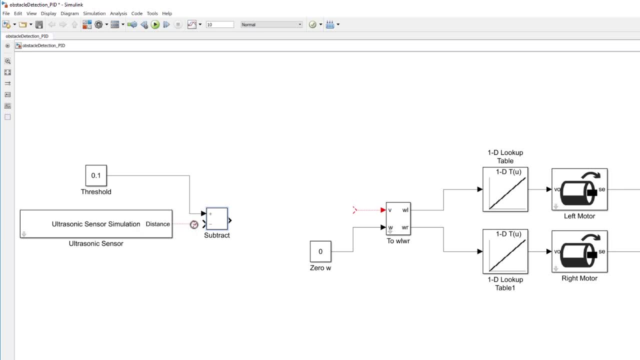 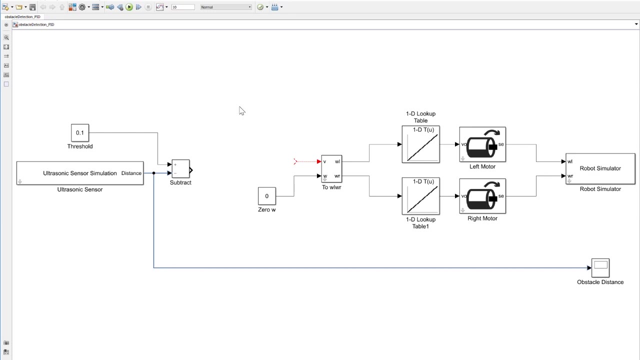 sign of the subtract block, and the actual value is the value given from the ultrasonic sensor. So let's connect that to the negative port on the subtract block. Let's also connect the output of the ultrasonic sensor to the obstacle detection scope. This will help us visualize the value Now. next let's add a. 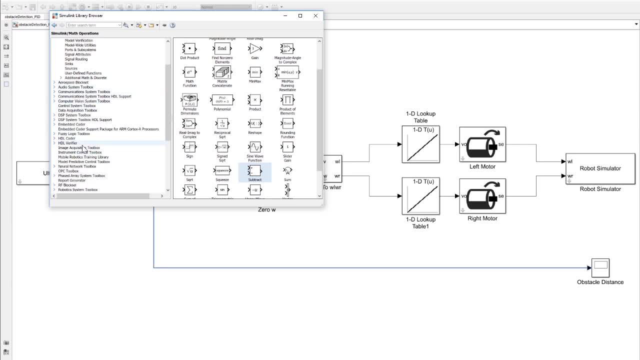 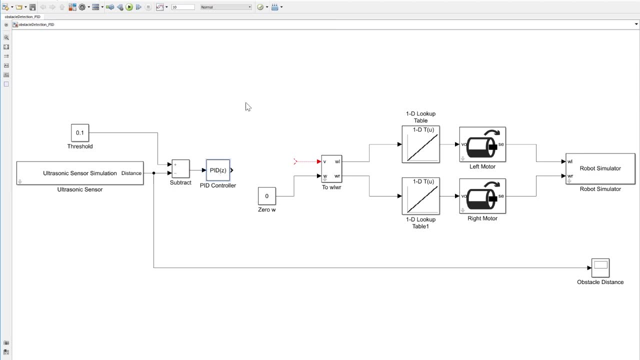 PID controller from the mobile robotics training library And let's connect the PID controller to the subtract block. The PID will output the V value for the robot, So let's connect it to the V signal right here. Since our robot is moving in a straight line, the Omega value would be 0 and that 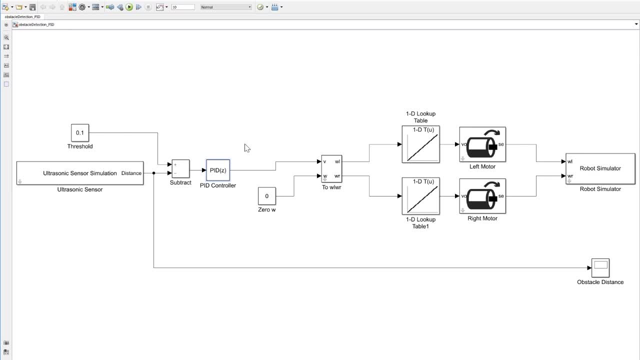 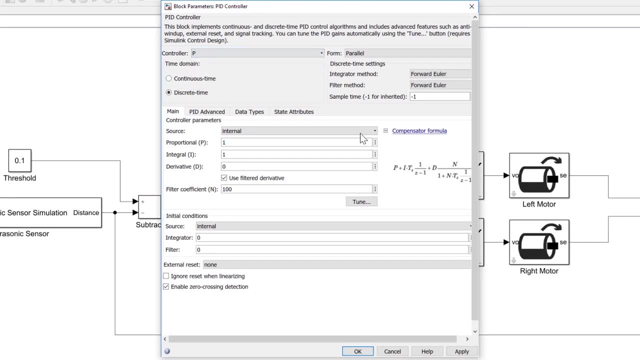 is given from the 0 Omega constant block. So now let's double click on the PID controller to set up its parameters. Let's choose the P only controller first and let's set its gain to 0.1 meters. Now let's connect the PID controller to the. 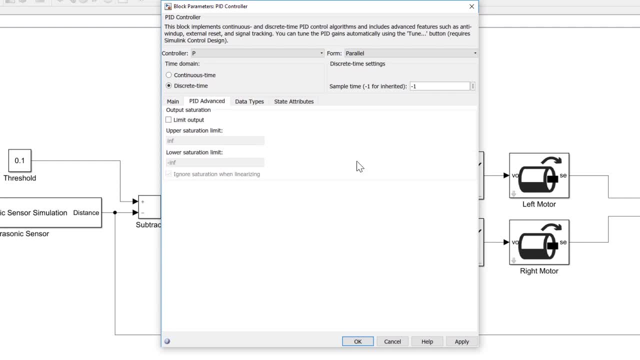 default, which is 1.. Now let's go into the PID advanced tab and set the output limits of the controller. So let's limit the output and recall that our controller output is the linear velocity of the robot and that is constrained by how fast your motors can rotate. We already calculated this value in the 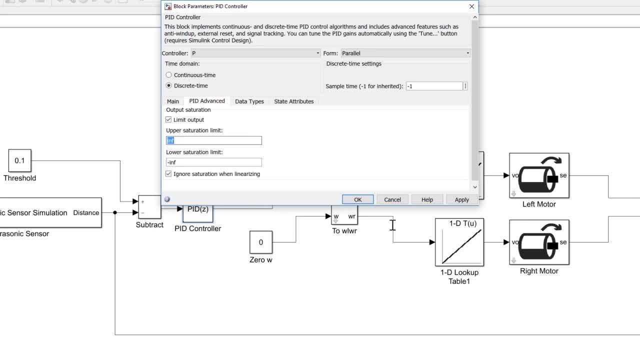 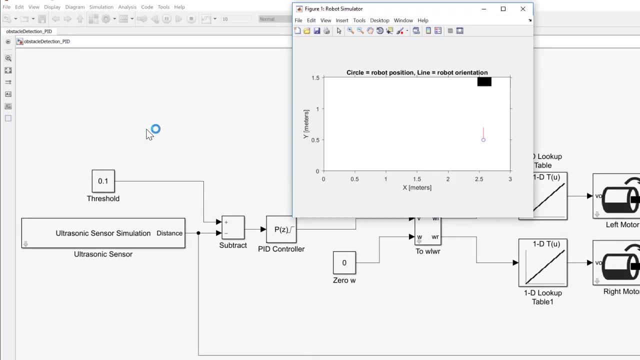 using PID controllers video- to be 0.67.. So let's set the upper saturation limit to be 0.67. And the lower saturation limit to be negative, 0.67.. Let's hit OK. And now let's run our model. We see that the robot is moving in the backwards direction instead of forwards. 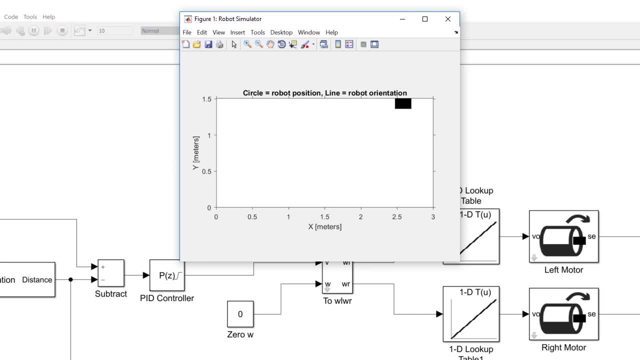 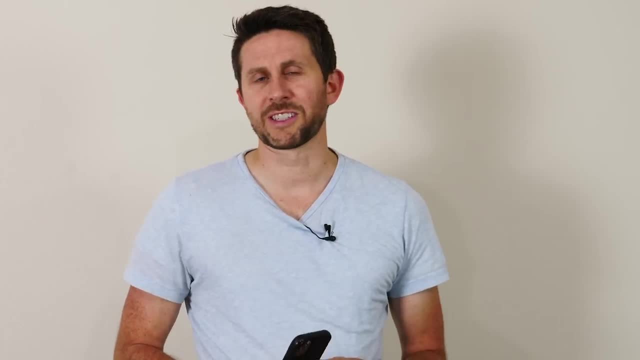 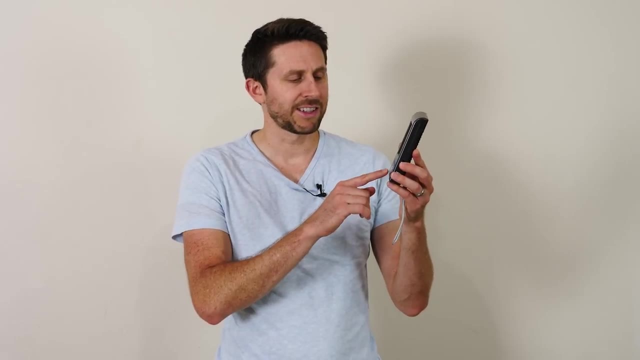 Hey everyone. today we're going to be testing if the 5G signal from your cell phone is going to kill you or not. In order to test this, I finally got my hands on a 5G radiation detector. This is called the GQ EMF-390.. I'll put a link to it in my description. 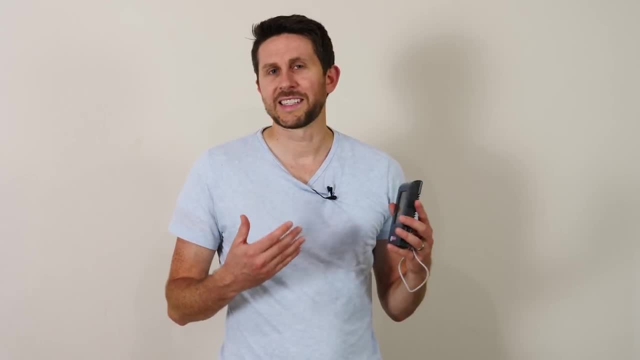 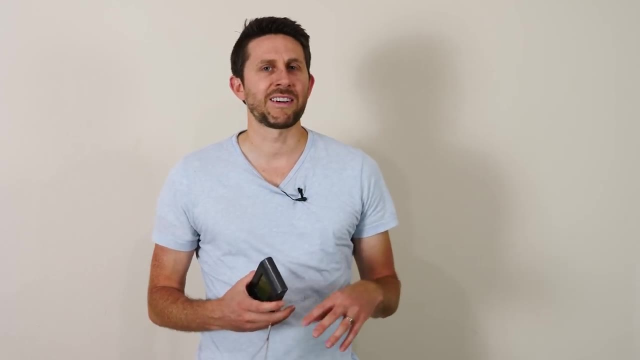 GQ actually sponsored this video and sent me this device so that I can test out the electronics in my house. So I'm going to be testing the strength of radiation that comes from my cell phone, also my Wi-Fi in my house and also the cell phone towers as well. 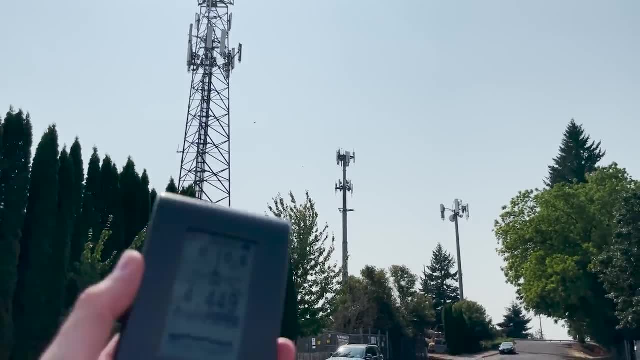 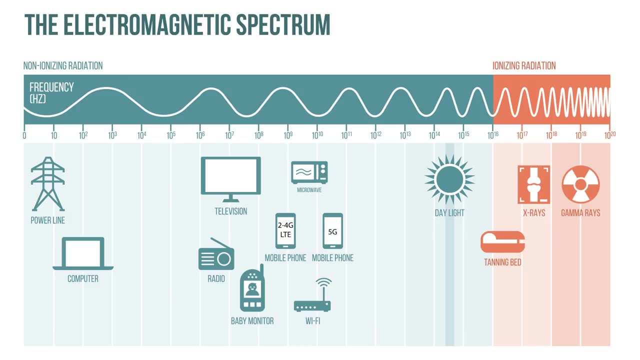 So I'm going to be driving to some cell phone towers and testing how strong the radiation is at ground level. The term radiation in and of itself doesn't actually mean something is dangerous. Electromagnetic waves come in all different ranges. You can have radio waves which have extremely long wavelengths. 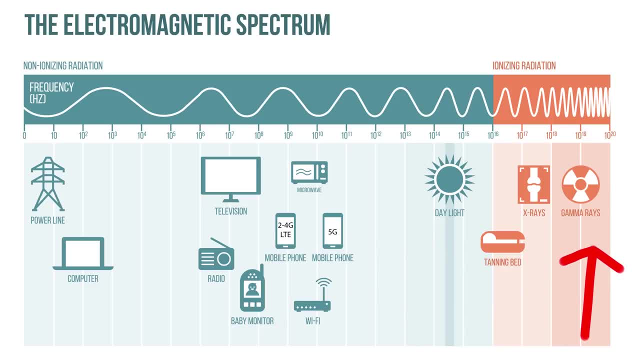 all the way up to gamma rays, which have extremely short wavelengths. Usually, the electromagnetic waves that we're worried about are the electromagnetic waves that have really short wavelengths, because that means they have a lot of energy, And when they have really short wave wavelengths,